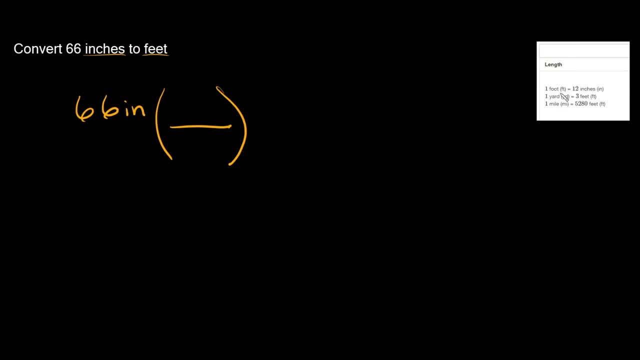 we're trying to convert from inches to feet, So you need to find a relationship between inches and feet And, as you can see, the top one gives us just that right. It says 12 inches is equal to one foot. Okay, so that's what we're going to fill in right here. Now do we put the inches on the top? 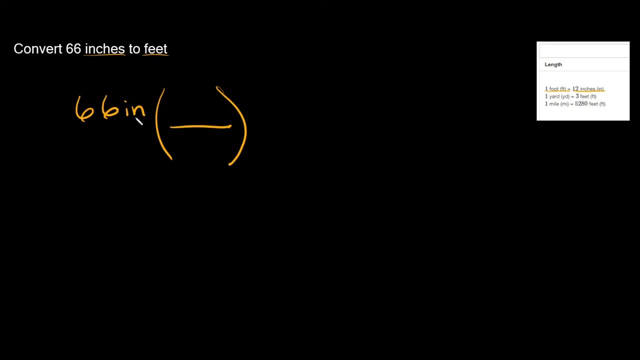 or the bottom. Well, the easy way to figure it out is: whatever units you have up here is what you're going to have in the bottom. Okay, so I'm going to put inches down here. Okay, so it's really important to make sure you never put the same units on the same. 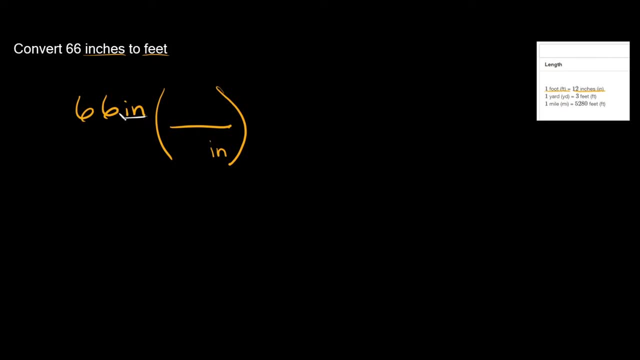 side. So, as you can see, we already have inches on top right here, right? That's why I cannot put inches on top right there. Okay, you always need to put it on the opposite side, which is why we put inches on the bottom, All right. so remember the relationship was: 12 inches is equal to one foot. 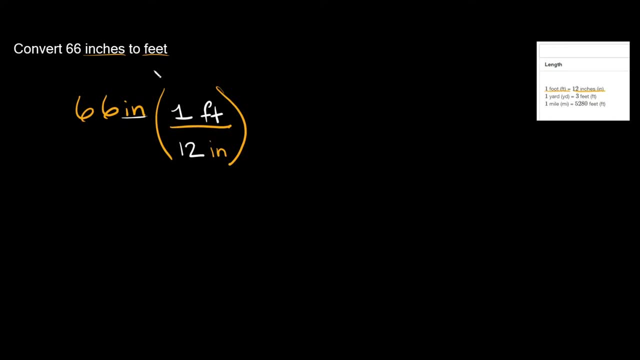 Okay. so, remember, we're trying to convert to feet right. So now that we have feet up here, now we can start canceling out our units. Okay so, since we have inches on top right here, that's going to cancel out with the inches on the bottom right there. Okay. so now you can finally simplify this. 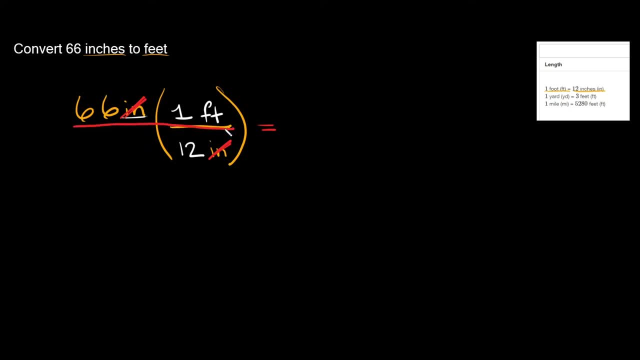 All right, so all you're going to do is multiply everything you have on top right here, So what we're left with is 67. And you're going to multiply that with one foot And that's going to go over whatever you have on the bottom, which we just have: 12 right there, right? 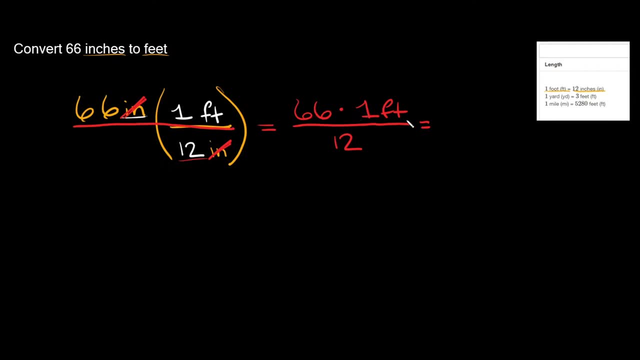 Okay, so simplifying some things: 66 times 1, that's equal to 66.. And then don't forget your units, right there: feet, That's going to go over 12, right? And then simplifying this one more time: 66 divided by 12 is equal to 5.5.. Okay. 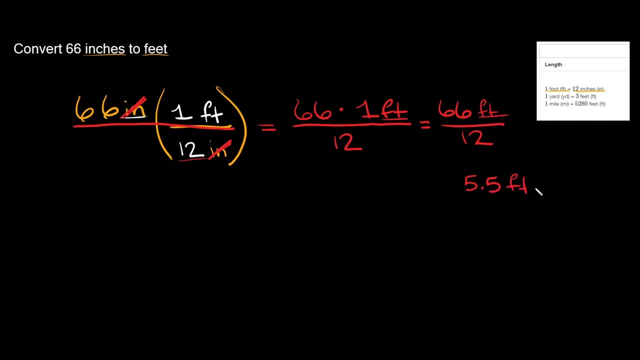 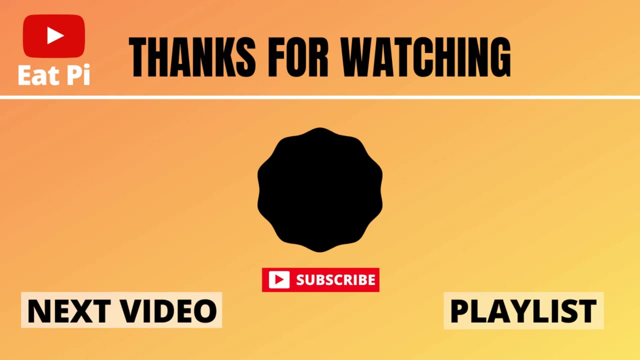 And then you still keep the units right. They didn't go anywhere Feet. So if you found the video helpful, definitely leave a thumbs up down below, And if you have any other questions or want to see any other examples, just let me know in the 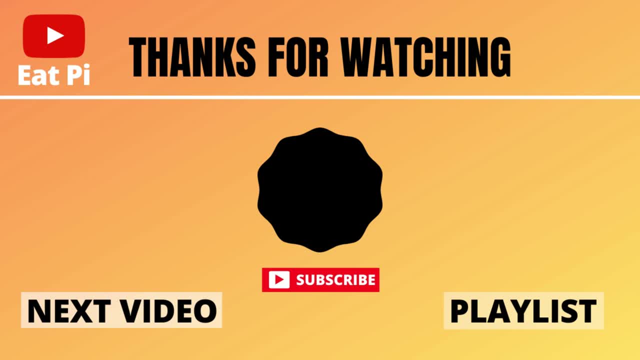 comment section below. Also, there's a couple playlists attached that I think you'll find helpful, So definitely check those out and I'll see you there.